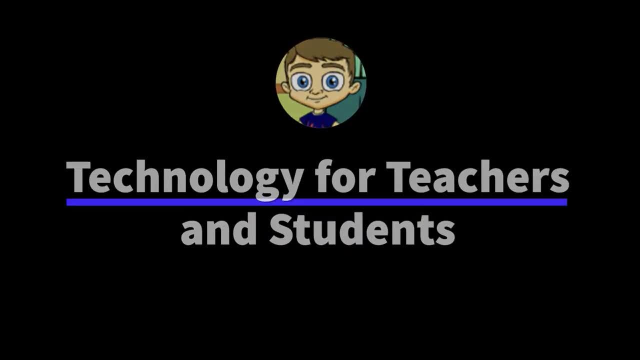 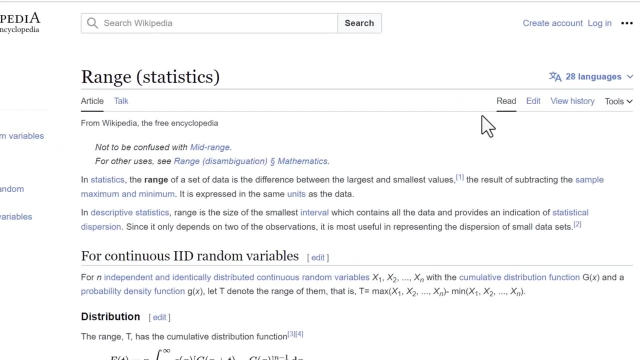 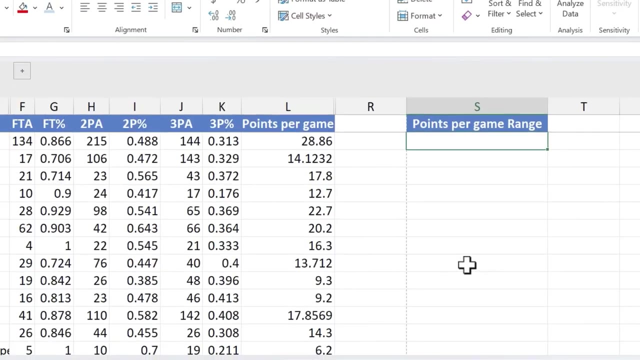 In this Excel video I'm going to show you how to calculate range in Microsoft Excel. In mathematics, range is a statistical term that means the difference between the largest and smallest values. So here in my spreadsheet I have a list of some NBA basketball players and I want to 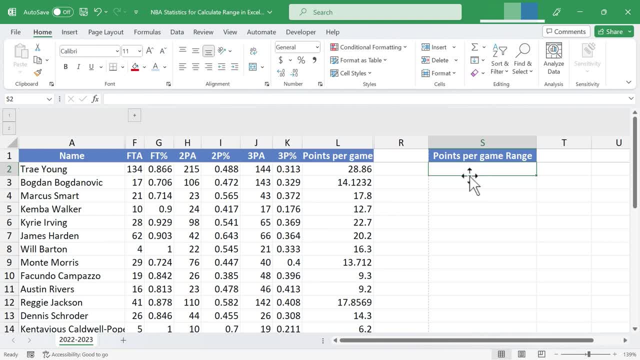 calculate the range of their points per game. To do this, I'm going to create a formula that uses two different functions, max and min, And if you want to learn more about max and min, please watch my other Excel function tutorials and you'll learn much more about them. But here I'm just 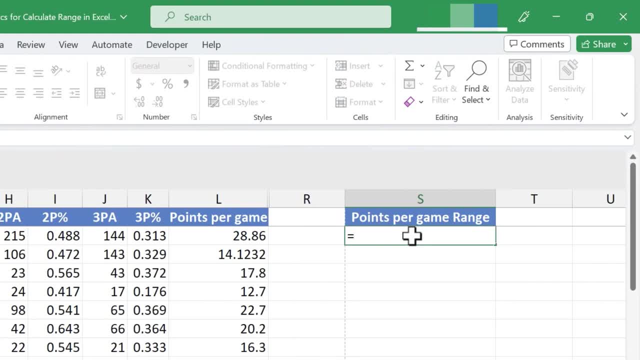 going to click on cell S2.. I'll type equals and then max. Then I'll put in my left parenthesis and I want to search for the maximum number, in other words the highest number in column L. So I need to select the data in column L. I could click and drag to select the data in column L. 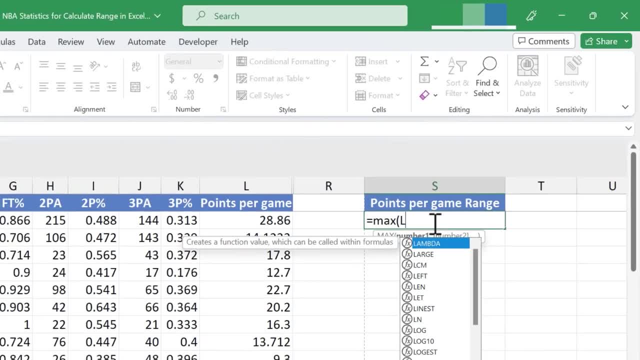 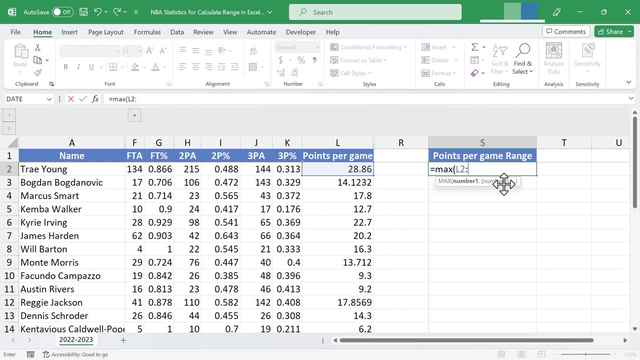 Or I could just type in the cell reference: So L2 through, and in Excel the way you write through is with a colon, So L2 through L30.. So I'll just type in L30,. put in my right parenthesis Now. I. 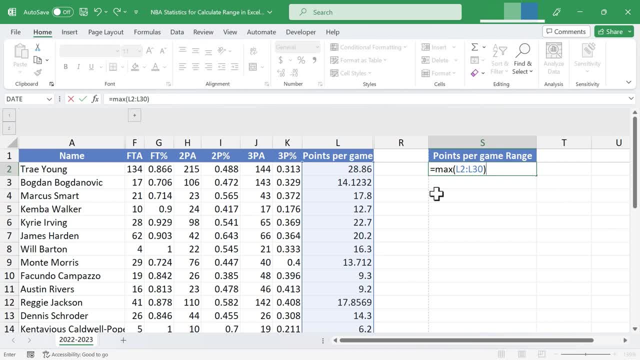 need to subtract the minimum of that same range, So minus min left parenthesis, and again I need L2 through L30.. I need to put in my right parenthesis and I need to put in my left parenthesis. Sometimes the right parenthesis is not necessary, but in this case you need it, So it's a good idea. 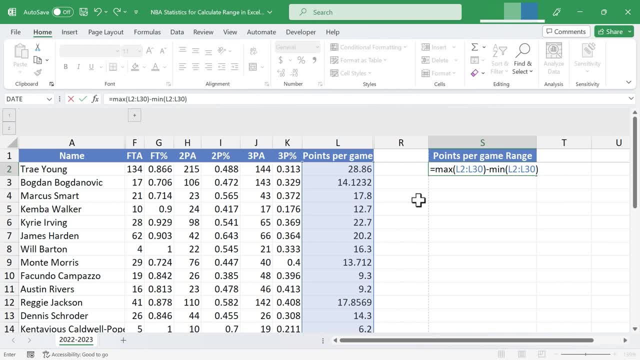 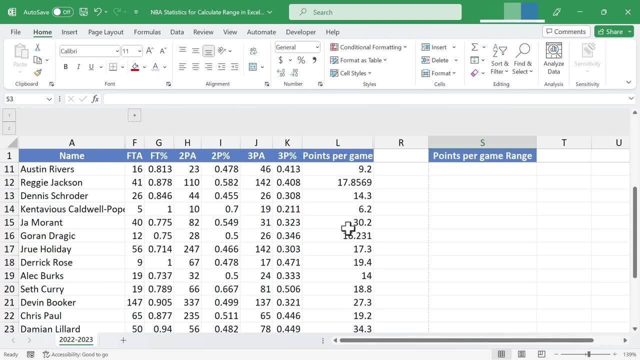 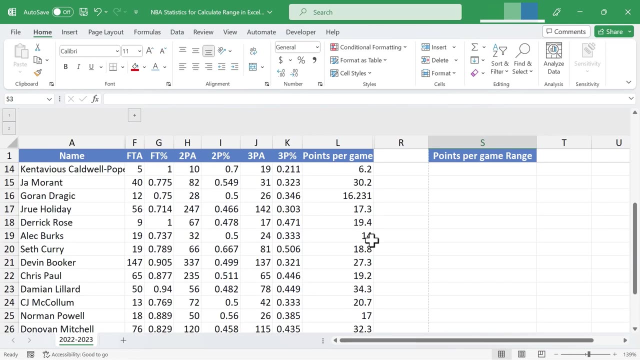 to kind of get in the habit of always putting in that right parenthesis. I'll tap enter on the keyboard and, according to Excel, there is a range from the lowest number in this group of data to the highest number of 28.1.. And just by eyeballing this I can see that that's accurate. It looks like. 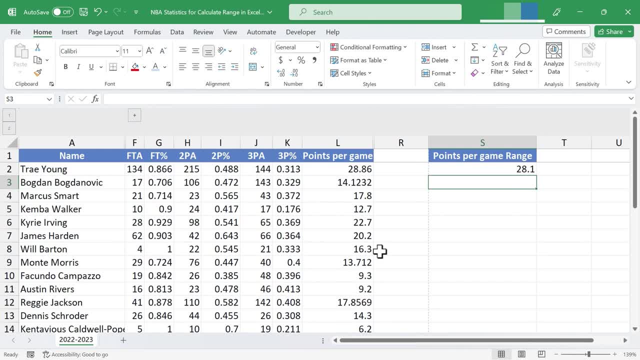 the lowest number is 6.2 and the highest looks like 34.1.. So I'm going to type in my right parenthesis And so that is a range of 28.1.. But imagine, instead of just 30 rows of data, what if I had? 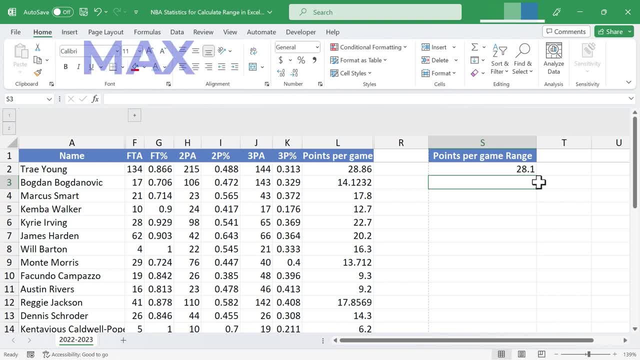 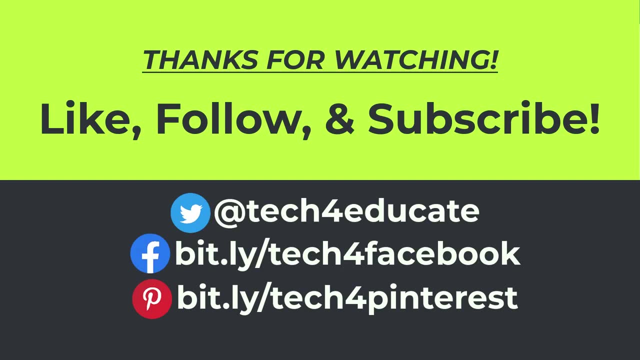 10,000 rows of data. Using this range formula that utilizes the max function and the min function, I can calculate very quickly the statistical range of a large group of numbers. Thanks for watching. I hope you found this tutorial to be helpful. If you did, please like, follow and subscribe, And. 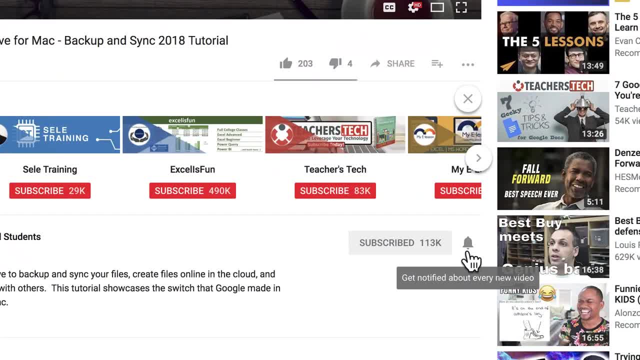 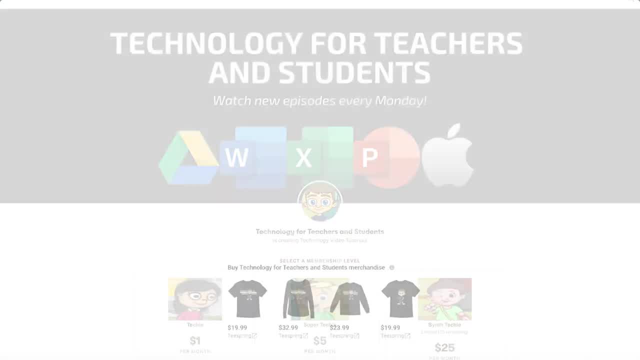 when you do click the bell and you'll be notified when I post another video. If you'd like to support my channel, consider clicking the thanks button below the video, And you can support me through my patreon account and by buying channel merch And you'll see. 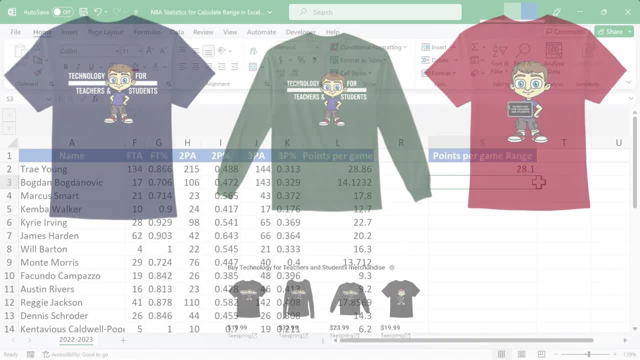 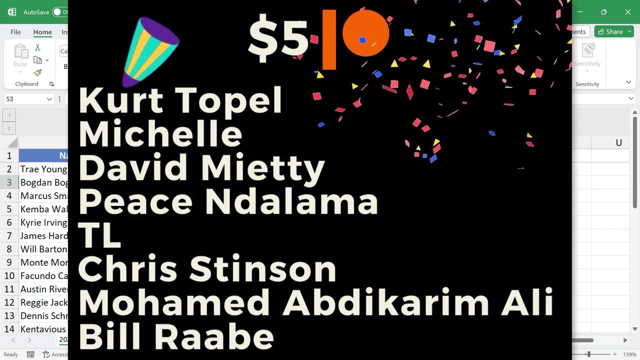 information about those options in the description below the video. Speaking of patreon, I want to give a quick shout out to my $5 patreon supporters. Thank you so much for all you do to support my channel. I really appreciate you. 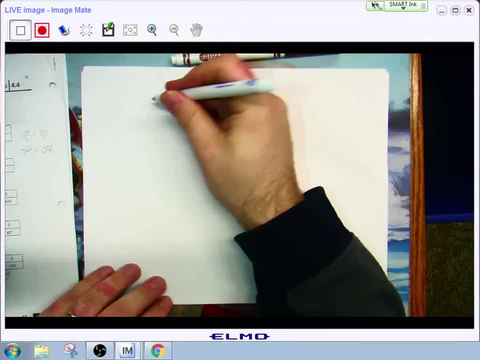 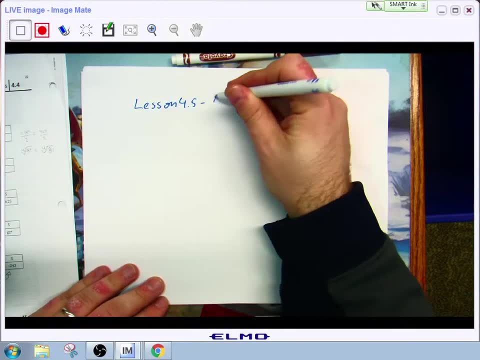 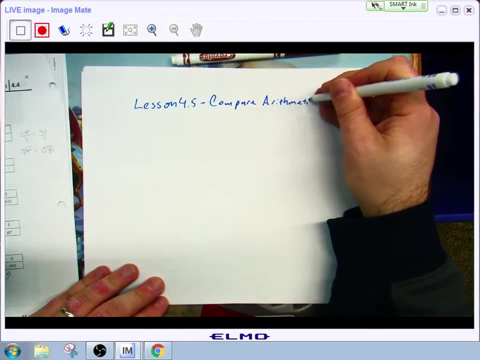 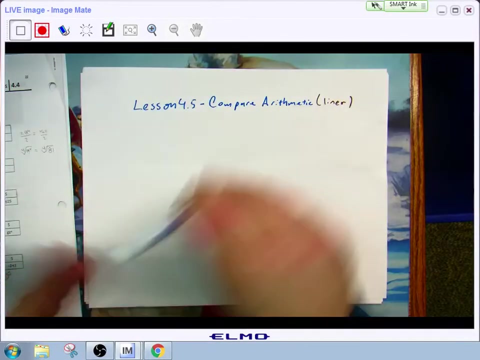 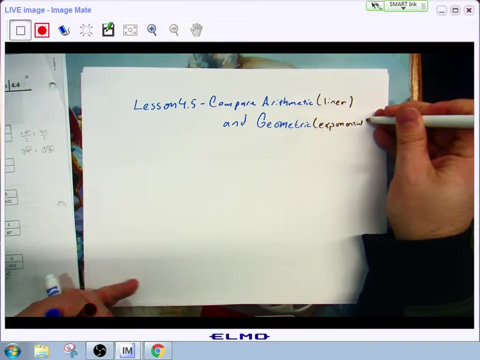 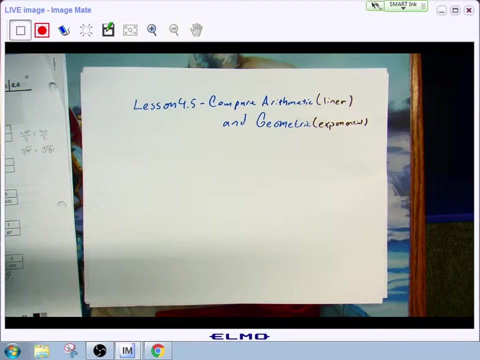 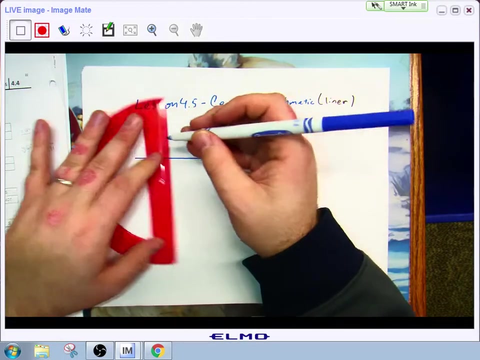 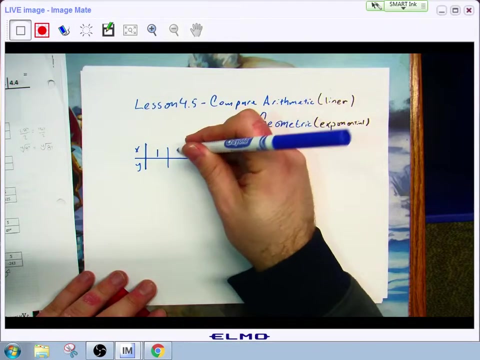 So this is lesson 4.5, and what I want to do is I want to be able to compare arithmetic, aka linear, and geometric. When we look at the second problem on our quiz, it looks something like this: We're given our x, we're given our y, we've got 1,, 2, 3, 4,, 5,, 6,, 7,, 8,, 9,, 10,, 11,, 12,, 13,. 12,, 13,, 14,, 15,, 16,, 17,, 18,, 19,, 20,, 21,, 22,, 23,, 24,, 25,, 26,, 27,, 28,, 29,, 30,, 31,, 32,, 33,, 34,. 35,, 36,, 34,, 35,, 36,, 37,, 38,, 39,, 40,, 41,, 42,, 43,, 44,, 45,, 46,, 47,, 48,, 49,, 50,, 51,, 42,, 43,. 52,, 45,, 42,, 45,, 46,, 47,, 47,, 48,, 49,, 51,, 52,, 53,, 54,, 55,, 56,, 57,, 58,, 59,, 51,, 52,, 53,, 54,, 55,, 56,, 57,, 57,, 58,, 50,, 51,, 52,, 53,, 58,, 51,, 52,, 52,. 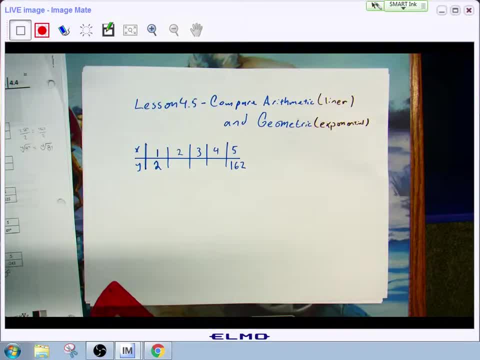 53,, 57,, 58,, 52,, 53,, 52,, 53,, 53,, 53,, 52,, 53,, 53,, 53,, 53, 52.. I asked you guys to find the missing values there. 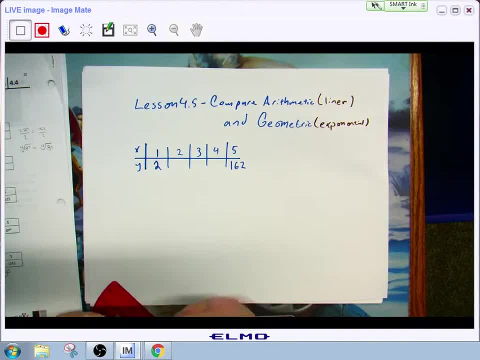 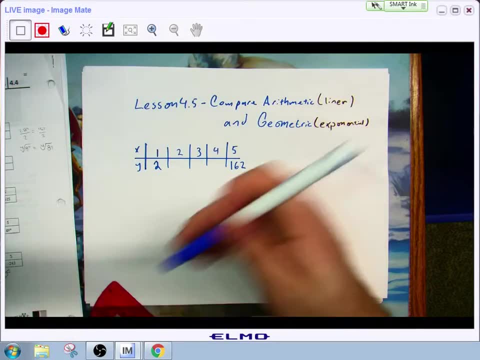 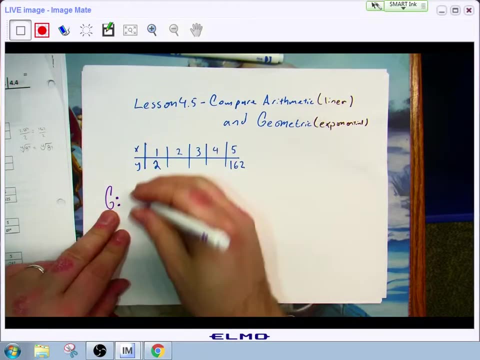 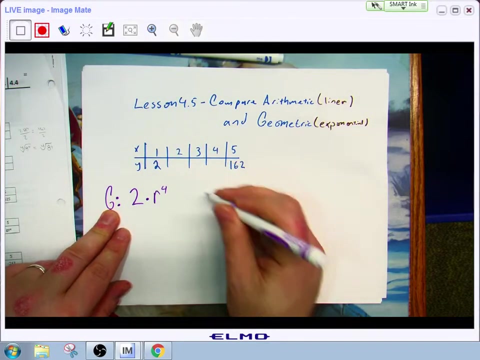 And so when you find those missing values, the problem itself asks for you to do it geometrically, And so the way that we've been doing this is that we've been looking at this and looking Geometric. I know that 2 times some sort of common ratio- 1,, 2,, 3,, 4 times r to the 4th power- is going to equal 162.